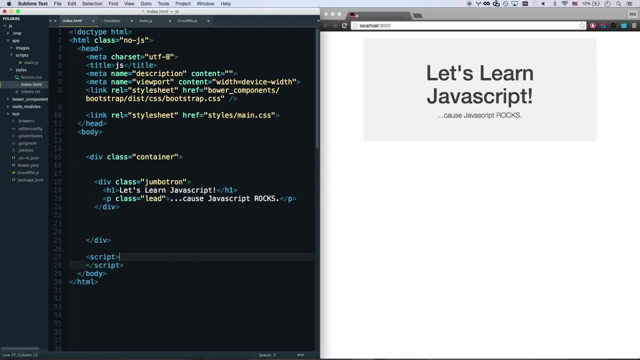 script tag And then anything within this script tag is treated as JavaScript. I'm going to say alert And I'm also going to hit save And I'm running what's called live reload. So when I save my file, this web browser is going to automatically reload my page, If 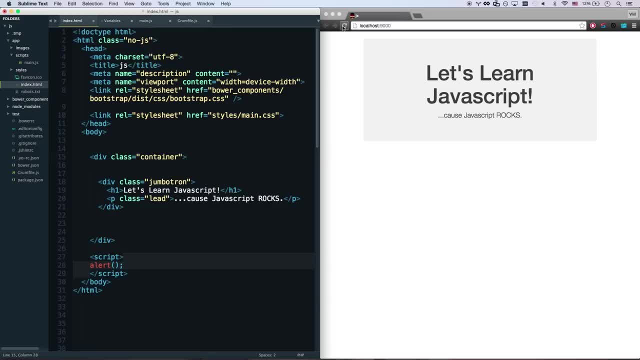 you're doing this on your own without live reload. you're going to have to save and then hit refresh. If you want to see how I'm doing live reload, I'll put some links to that in the description, But it might be a little over your head if you're a brand new user. 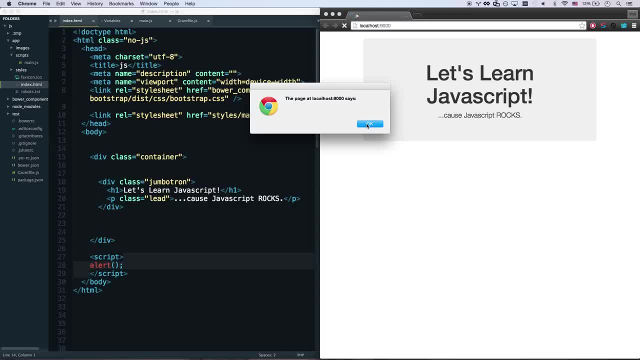 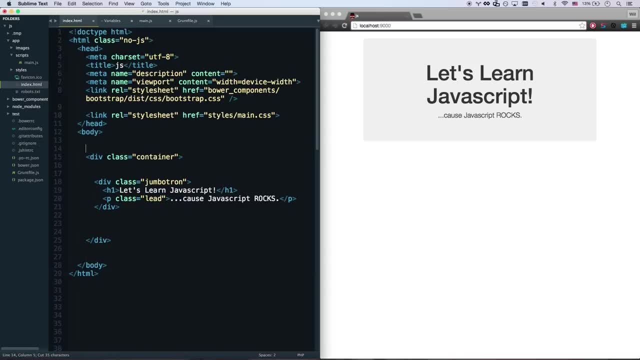 So there you go. You can see that now my web page, when it reloads, has alerted an empty alert for me, And there's a reason. I put the script tag at the bottom of the page, And let me show you why by moving it up towards the top. 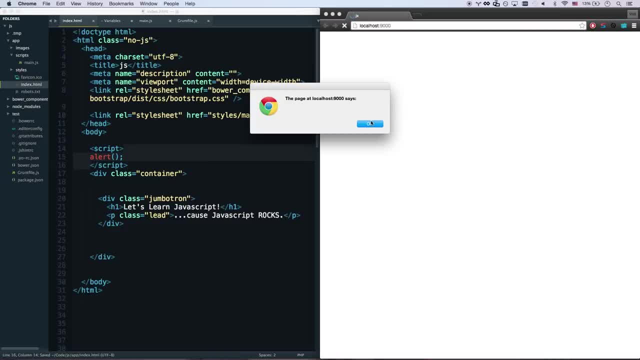 I'm going to hit save again And you'll notice that now I get the alert before I see my web page. I have an empty page and the alert fires. This happens because JavaScript happens in sequence as your web page is rendering all the elements. What that means is when your 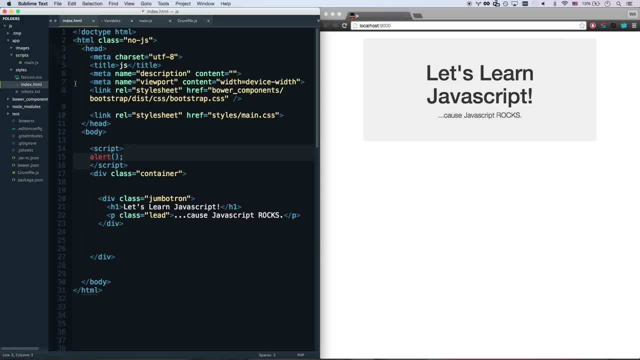 browser opens up your HTML site, you're going to be able to see the elements that you're HTML file. it's going to start going through line by line and adding in all the elements. So when it gets to a script tag, it's going to load all that JavaScript and then it's. 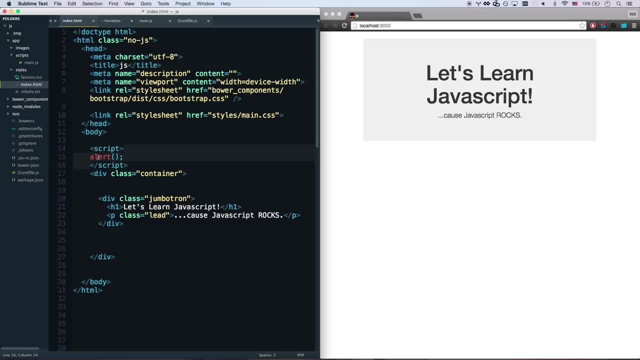 going to run it before it does anything else. So in this case it runs my alert up here before it's rendered all these elements onto the page. You know, JavaScript is really pretty fast. You're not really doing alerts a lot, So all. 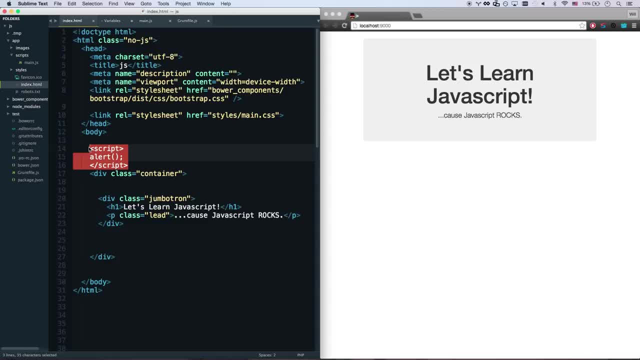 the user will normally notice if you put your script at the top of the page is the webpage might feel like it appears a little bit slower. If you put it down here at the bottom of the page, right before the closing body tag, then what's going to happen is is your webpage. 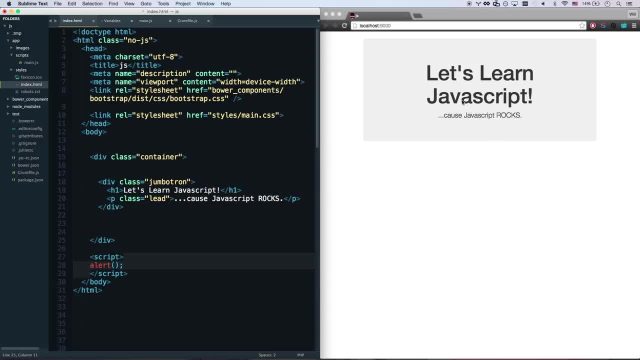 will spit out all the content first, so it looks like the webpage is loaded and a split second later your script will be activated And web developers have learned over the years that this creates a much faster feeling webpage and the user doesn't know any different. So 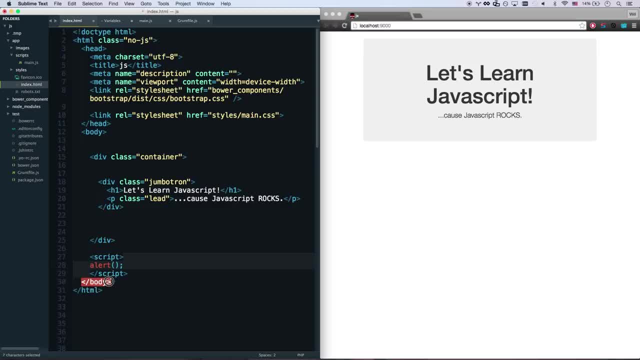 we recommend that you always put your script tags at the bottom right before your closing page. There's almost never a reason that your script needs to go in the top up in the header. So the script tag is the first way of doing it And, just like a link tag, you can also give. 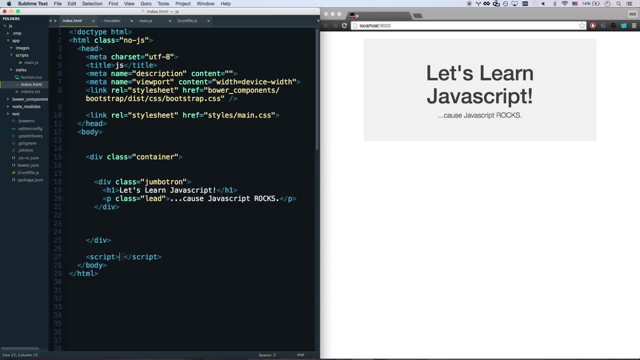 the script tag, a file to pull in as well. So in this case I'm going to delete the content and I'm just going to go source: SRC equals, and then that basically is like the href is for CSS. So instead of pulling in the styles maincss, I'm going to pull in the scripts. 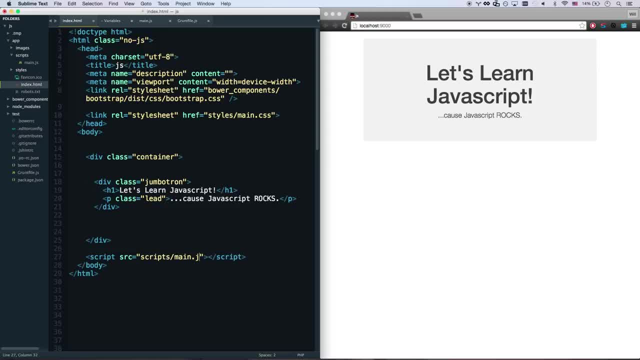 mainjs, And now that file gets loaded in and executed. as soon as it's loaded, The normal folder name for JavaScript is going to be called a js folder or a scripts folder. So here we have. scriptsjs is just fine, Either one works. So now I'm loading in this mainjs file. So 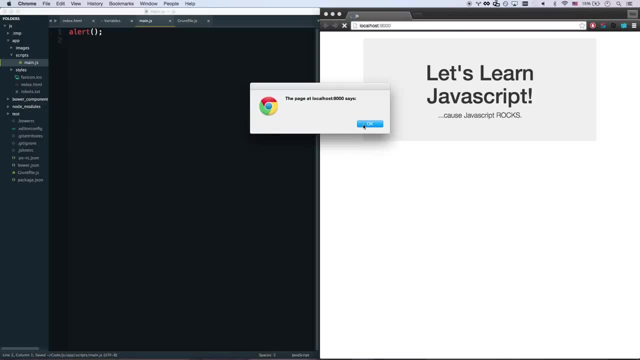 if I hit alert and save, you see, I get that alert as well, and it's already rendered my webpage first before it's executing my JavaScript. So there's how you get JavaScript on a page. If you have multiple JavaScript files, you can do multiple script tags, just like that. 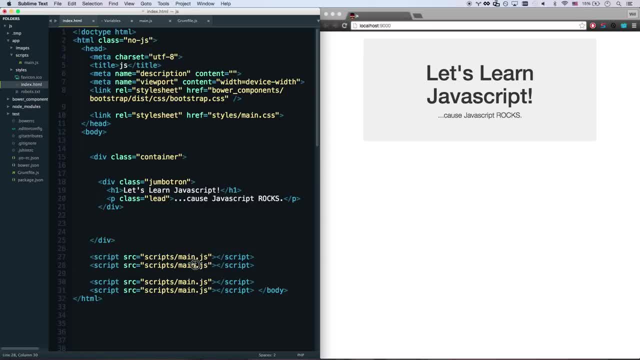 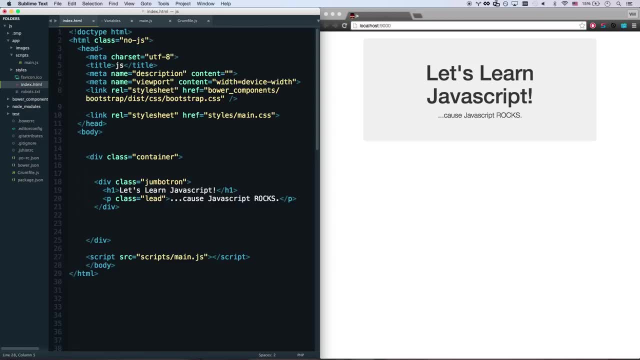 and it will execute them in order. It's going to run my mainjs first, then my main.2, then my main.3,, then my main.4.. So that's what's going to happen if you have multiple script tags, if you want to break up your JavaScript into several files to make it easier to maintain. 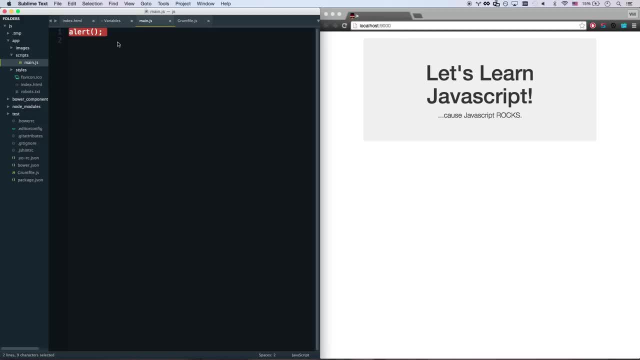 So let's go ahead and learn about functions. So functions are basically a piece of code that does one or more actions. Piece Of code that does one or more actions. So I'll just show you what a function is, because it's a lot easier to see it than to hear about it. You start off by typing function and we'll 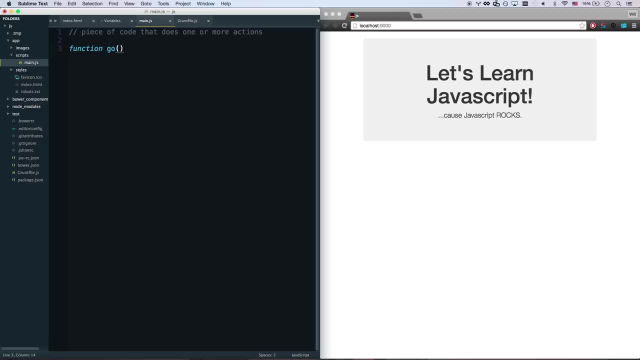 just call this function go. You open and close your parentheses and then you open and close your curly braces. So whatever I put in here is going to execute when the go function is called. So let's just say alert, hi, Alert, hey there. 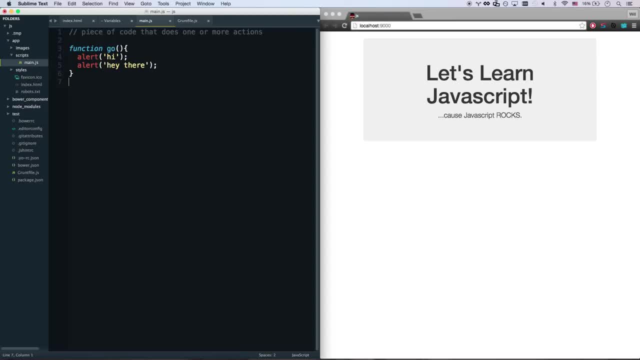 And so it's going to do two alerts. I'm going to save my web page refreshes and guess what? Nothing happens. because I defined my go function but I didn't call my go function. I call it by saying go open and close parentheses and then a semicolon. Now, when I refresh, it's. 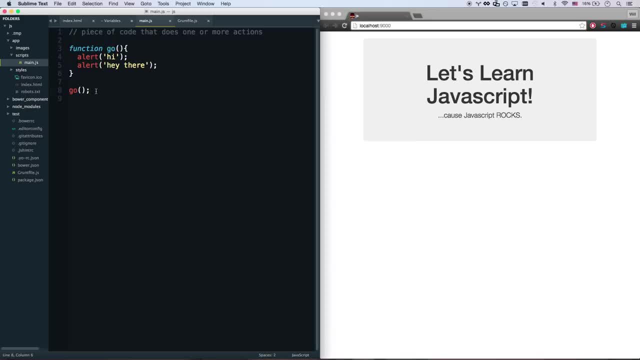 going to say hi, and then it's going to say hey, there, I have my function. A cool thing about functions is they can be called as many times as you want. I can call go twice. Hi, Hey there, Hi, Hey there. 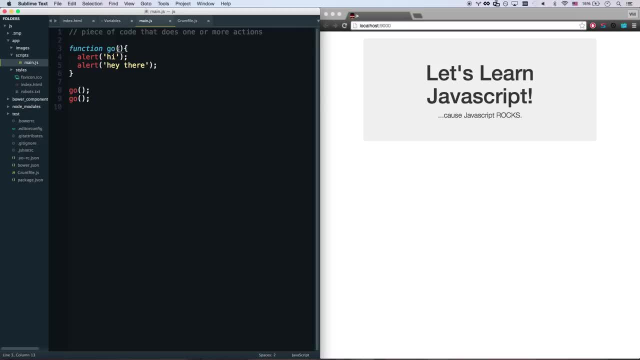 Hey there. So that's kind of cool. Another thing about functions is they accept what are called arguments. Let me show you what arguments are. I could say name, age and then instead of alerting hi, hey there, I can alert name and I can alert age. Now in. 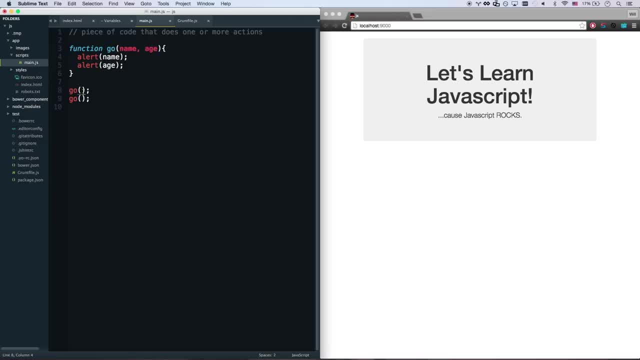 order for it to know what the name and the age are, I pass them in when I'm calling my function So I can say my name is Will and I'm 34 because I just had a birthday. So now Will gets passed in as the first argument, which is name, and 34 gets passed in as the 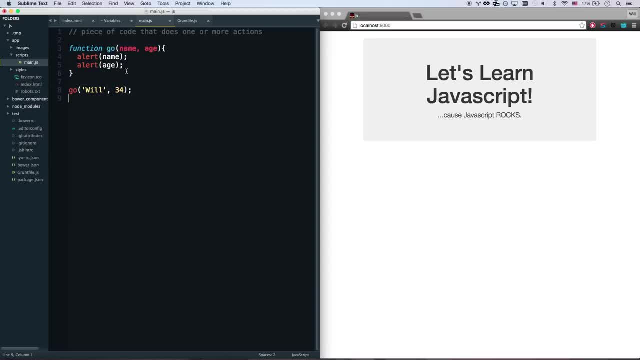 name. So that's kind of cool. So that's the way you can do that. Let's go ahead and show you some processing. passed in is a second argument, which is age. so now it's going to alert will and then it's going. 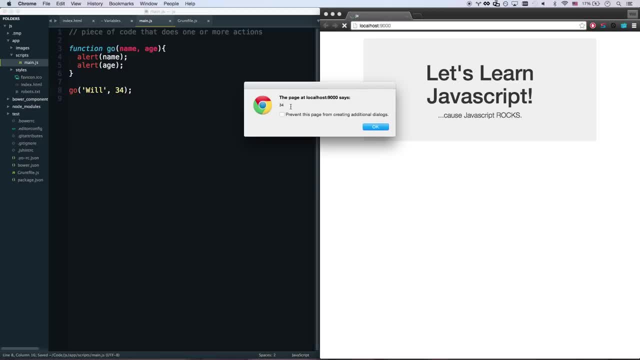 to alert 34. let's save it. there you go will. there you go, 34. once again, these are called arguments. and what arguments allow us to do? is they allow us to make code reusable, because at first you might think, hmm, i could just stick to go. i could go. their name equals will, and then their age equals. 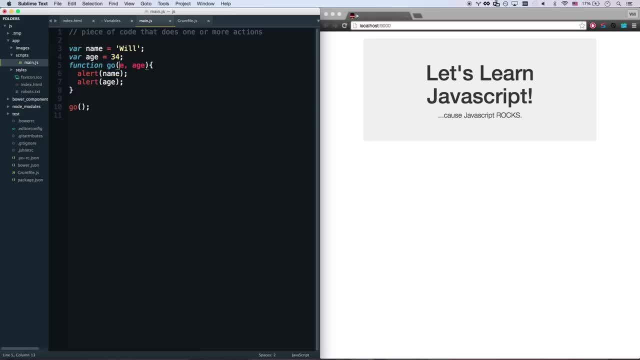 34, and then i could forget this whole arguments thing and i could just say: alert name age. well, yep, that's going to do the same thing, it's going to alert will and it's going to alert 34, but if i code it with arguments, it's reusable. let me show you. let's go back to name age. let's go back to. 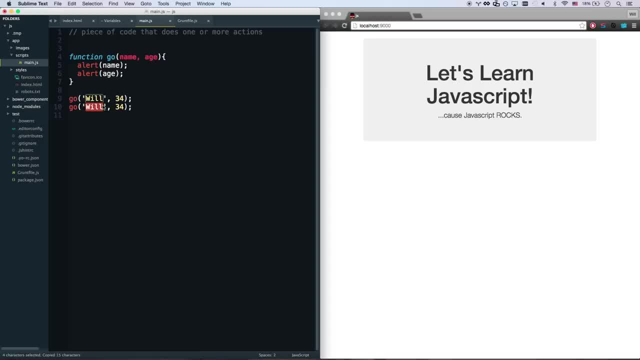 will 34, and now i can call it a second time with a different person, let's say my wife laura. 28, 28, 28. there we go. so now it's going to run one time with will and 34 will 34, and then the next time. 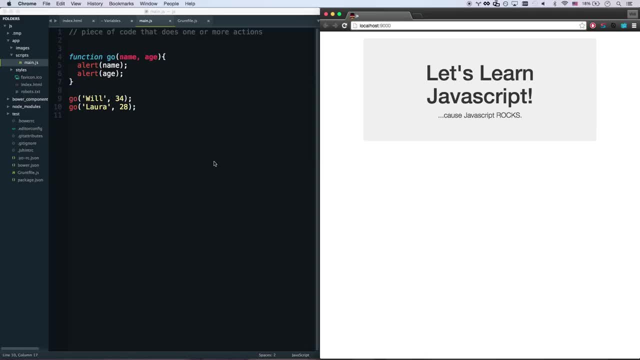 it runs. it's going to run with laura 28, and so that's kind of a good way of coding it's. it's called dry, which is do not repeat yourself. if i could spell, do not repeat yourself. d r? y, do not repeat yourself. or don't repeat yourself. 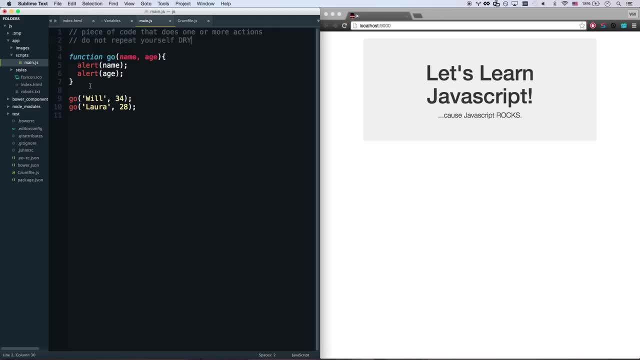 so dry code is a good thing. we want to code as little as possible. that makes it easy to maintain, that makes for as few lines of code as possible. so that's kind of what a function does. it accepts arguments and it runs multiple commands. now, a function also returns a value, whatever you type. 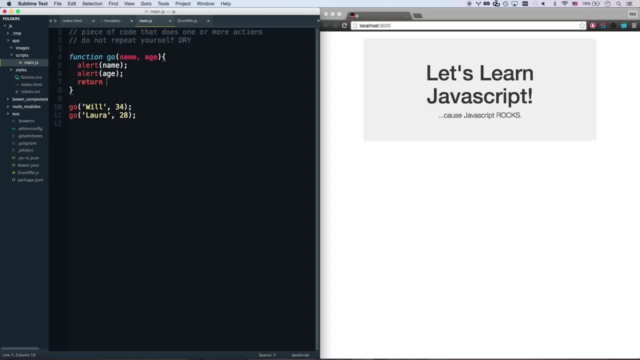 in return will actually give you a value out. let me show you what a return value does. you might remember from prompt earlier in the first lesson we went: var name equals prompt and then prompt opened up a window. well, i'll just show you right there. it opened up a window. and then, when i said 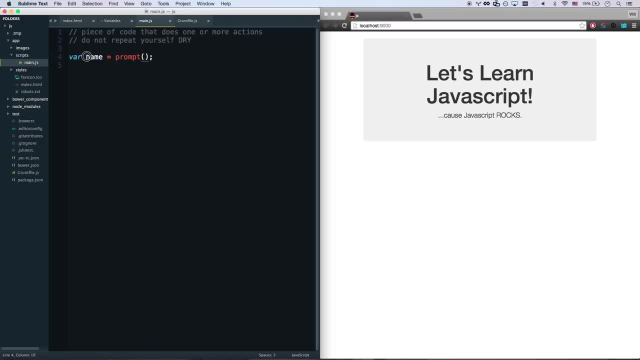 will enter will got passed in from the prompt into my name variable. so what actually happened was: is prompt had a return value that name received. you see that it executed this first and when prompt was done, whatever prompt returned which was my name will, went into name. and so how you code a. 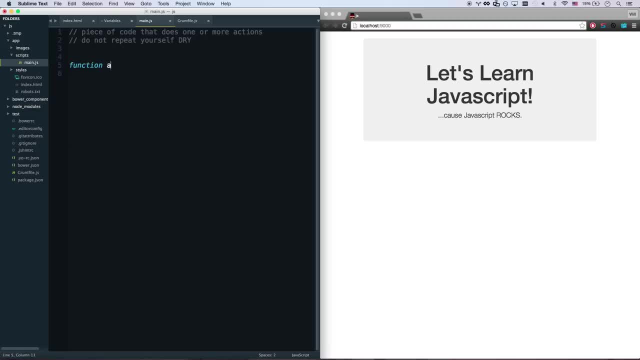 function like that is very simple. let's make a function called add, and let's make it first. second, we want to add two numbers together, and so i'm going to go add. let's say var sum equals, add one and two. so we're going to add one and two together, and so instead of just going, 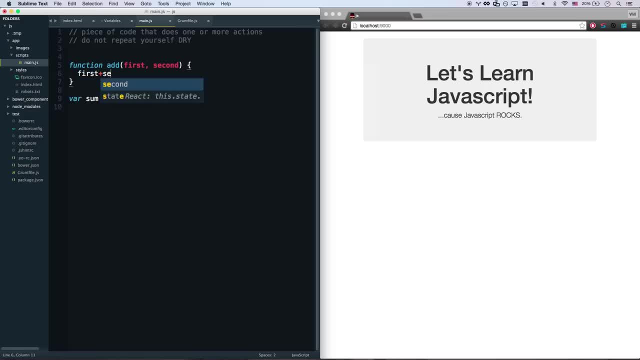 you, you first plus second. i'm going to return first plus second. so now nothing actually happens in this function like alerts or anything like that. we are going to return the value of first plus second, which means it's going to run the function, the function executes, it returns, kicks back out first. 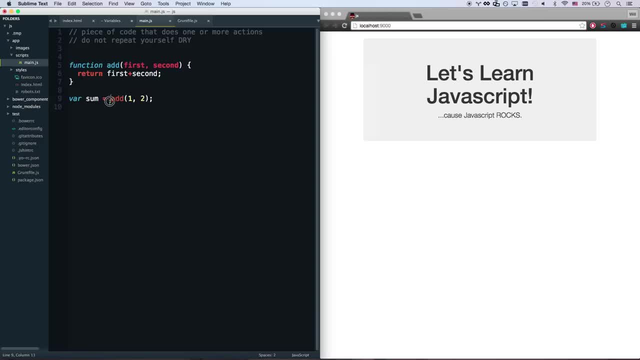 plus second, which means that it's going to add one and two and then that is going to get passed into sum. so now i can alert sum and sum is going to be three. there you go three because i added one and two. it returned that back out, so i could do something silly like this. i could pass in add. 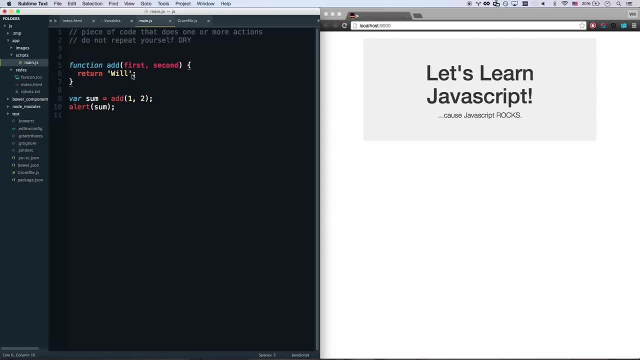 one and two, that's one, that's two. i'm just going to return will. so now it's just going to say, well, sum equals will, and i alerted two. i basically ignored my arguments. i returned whatever value i wanted to return, which is going to be one and two, and i'm going to return will and i'm going to. 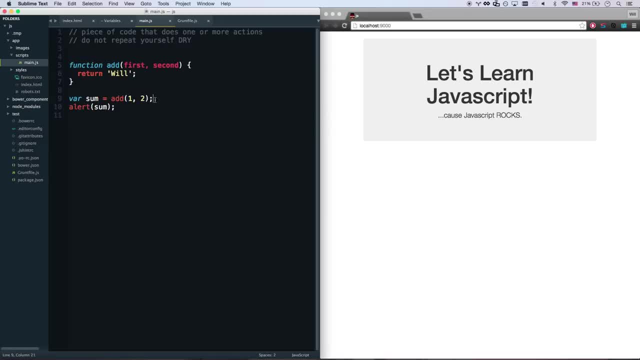 return one and two, which didn't make any sense, and that value got passed into here. so now now, no matter what i pass into add function, it's always going to return will, of course again, that's kind of silly. i want to return one plus two, and now i have my add function, another way that you can do. 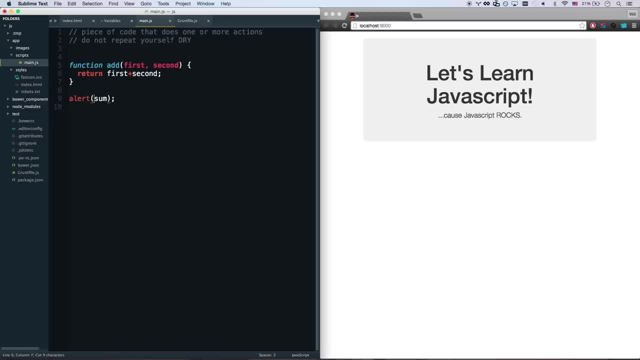 this with a little bit less code is. i could just alert, add one and two. so it's going to run this first because this is an inner function. javascript is going to know i have an inner function and i'm going to have to run this in order to know what to give to alert. whatever this returns, i'm going to. 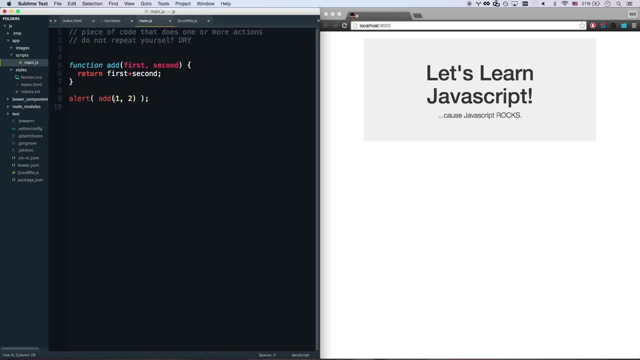 pass into my alert function as the value. so this will do the exact same thing. it's going to run one and two. one and two returns three, and then, as far as javascript is concerned, it's just going to alert that returned value. so i'm gonna save that. you see, it alerts three. let me show you what. 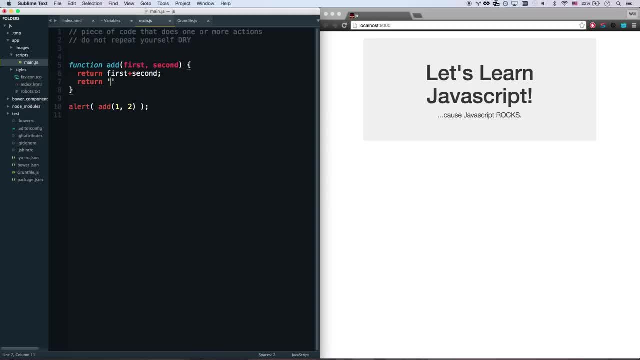 happens if you alert, if you return a second time, let's return will. now it does absolutely nothing because as soon as the return happens, this function is finished. what happens after the return? never fires. javascript is done, so i can say: alerts hi there and you're never going to see alert hi there. it alerts three from down here and i never. 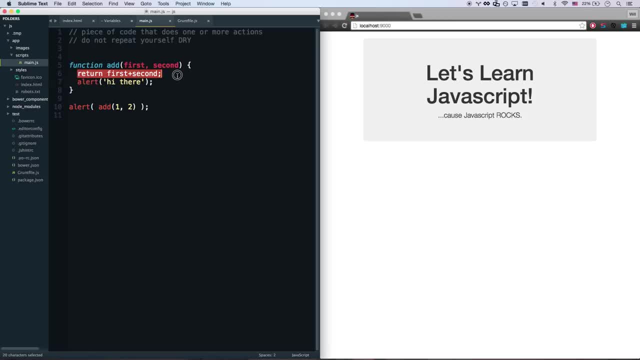 see the alert hi there up here. the function ran, it returned and then the function was finished. now you can have multiple returns. you could do something like this. you could do something like: hmm, let's go. ver. name equals. i will say this: um, let's go alert. 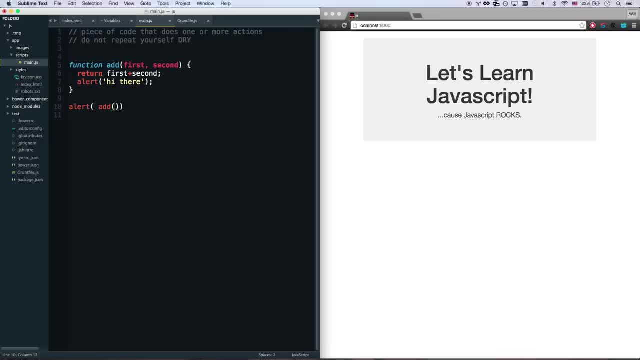 add. add is kind of a bad. we'll call, we'll go back to go, since we're not going to be doing adding will, and we'll go back to my, my age of 34. so this is going to be now called go name age. if age is less than 20, then we are going to return name plus an exclamation mark, because, after all, 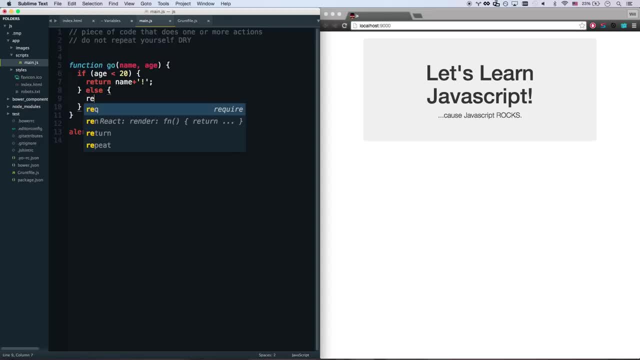 i'm less than 20, that's pretty cool, else we are just going to return my name. so now this will return a different thing. if my age is less than 20, then i'm going to return name shouted, else i'm going to return just my name. 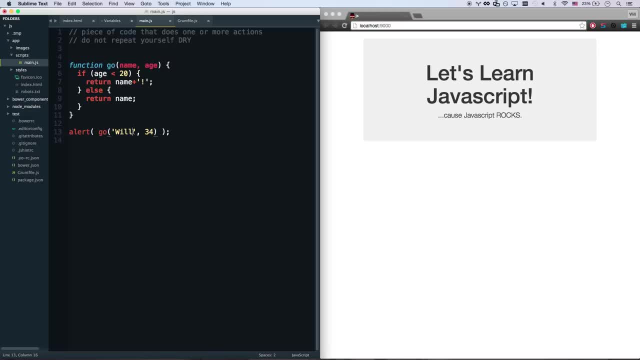 so go now, we'll check this out and it's just going to return my name because i'm older than 20, and then i'm going to alert that. there you go, just will. so let's change my name to 19, and now it's going to shout my name because, after all, you shout at teenagers a lot more than you do. 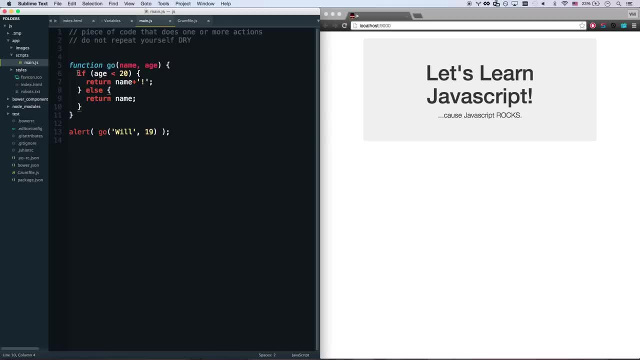 at adults. um, and what happens if i don't return anything at all? let's say, i say go name and age and i'm going to get undefined. so this function has no return, which means it's returning nothing, which means it's returning undefined, which brings us to one more of our types in javascript, and that. 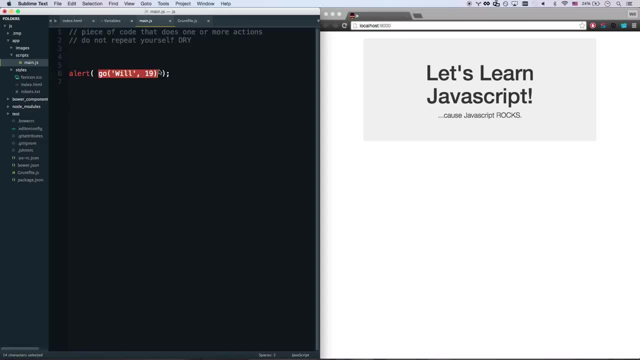 is the undefined type. if i say var a but i don't give it a value, then i alert a. it's going to alert undefined. i defined a as a variable, but i didn't define the value of a, so another type in javascript is undefined and it means simply well, undefined. so that's about all you need to know about this. 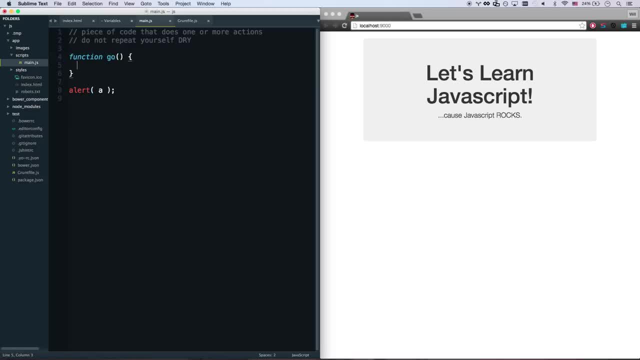 so by default, every function is going to return undefined unless you give it a return value, will again. so there you go. that's functions, let's um, let's leave it there for now. so i'm going to say: go ahead, make an addition function, make a subtraction function, make a multiplication. 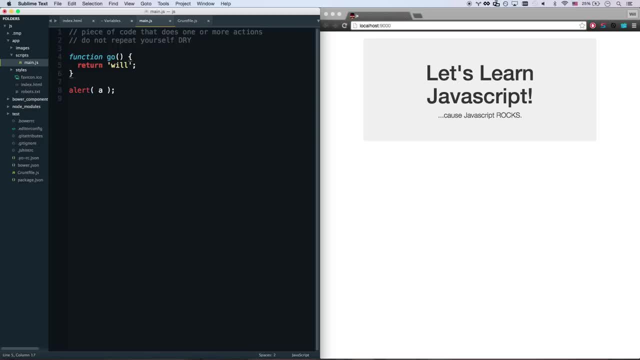 function, make some functions play around with them, and once you feel confident with that, let's move on to our last lesson before we get into some actual useful things. so let's get started with some useful things that we can use javascript for on our web page.